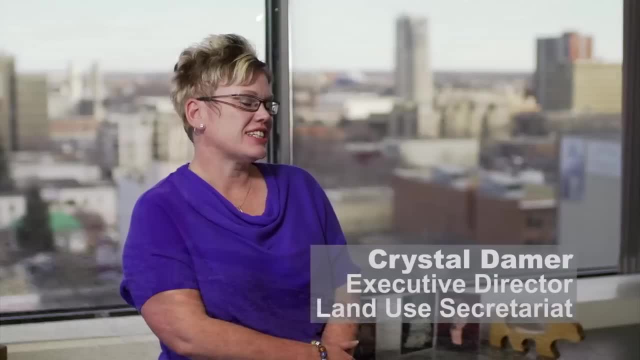 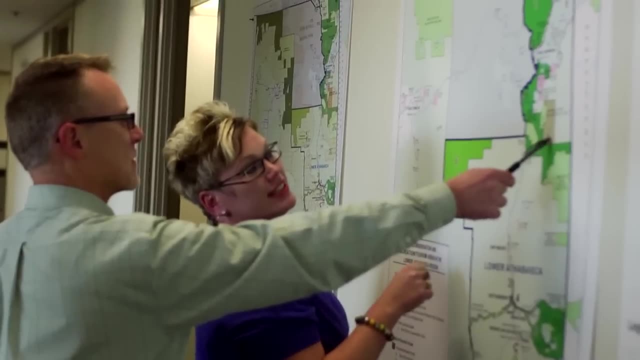 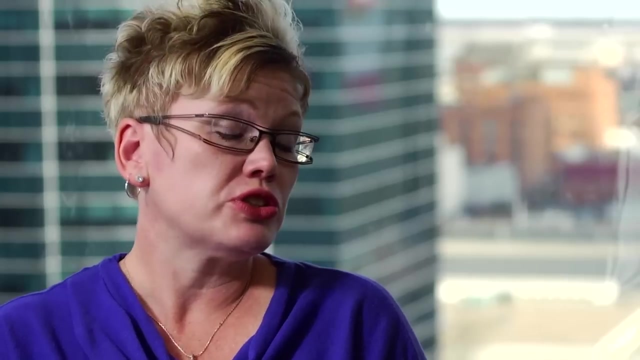 I'm Crystal Dahmer. I work with the Land Use Secretariat. It's a group of people- about 15 of us- that work on land use planning for the province of Alberta. Integrated resource management is about managing our resources. Alberta has an abundance of wealth in our resources from oil, gas, forestry, agriculture, rec and tourism. that all take place on the landscape. 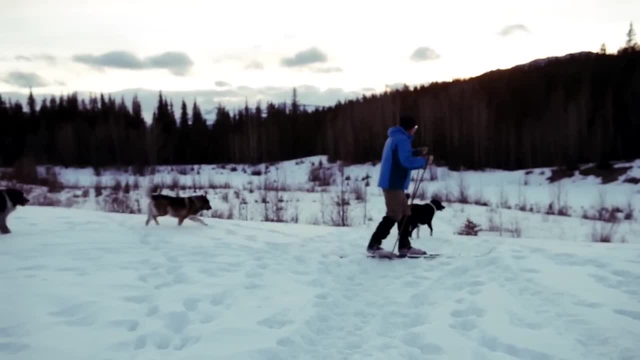 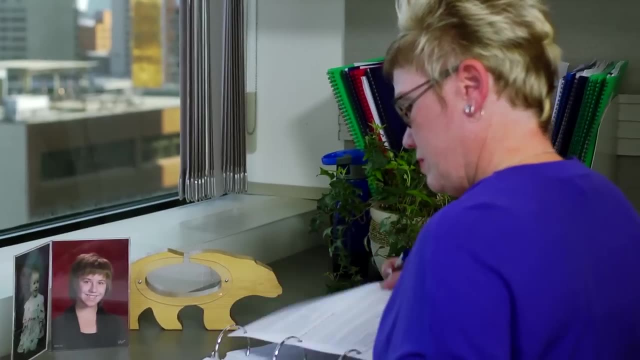 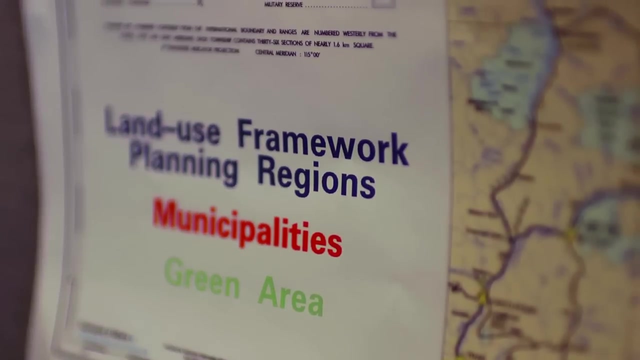 Albertans should care about land use planning and understand the importance of it, because it is planning for the next 50 years. It is planning your province. The province is based on seven regions that are based on watersheds. The regional boundaries are close alignment, as best fit to municipal boundaries. 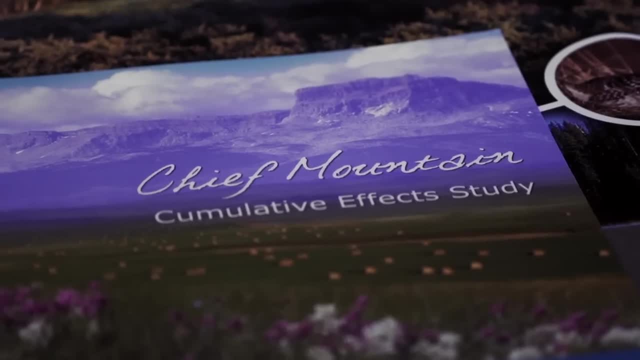 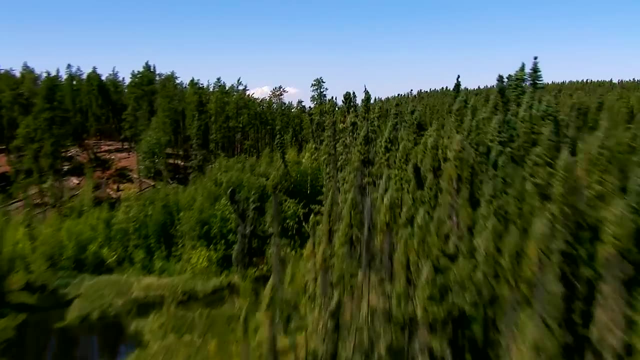 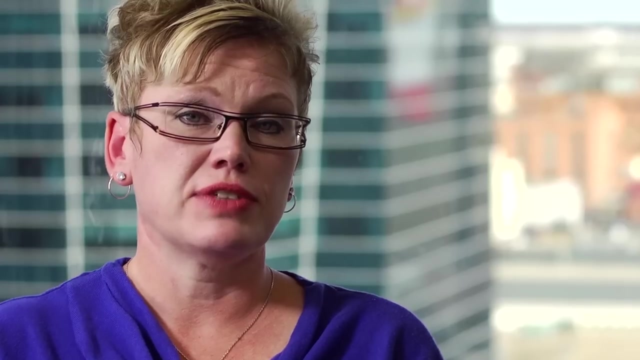 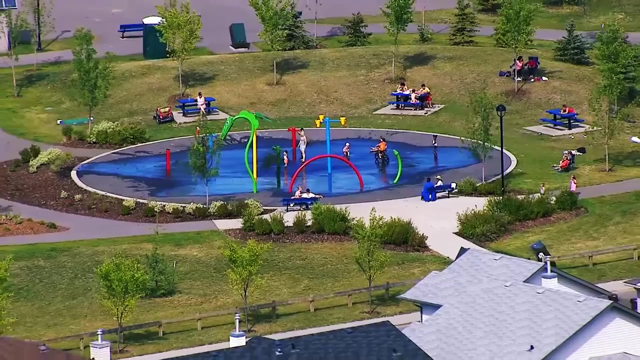 The process for developing regional plans is built to be transparent and we want everyone to engage with us throughout the process. The Lower Atholabasca Plan was the first plan developed under the Land Use Framework. It's an interactive plan. It's an area of intense activity. with oil sands development. It is the economic driver for this province as well as Canada. 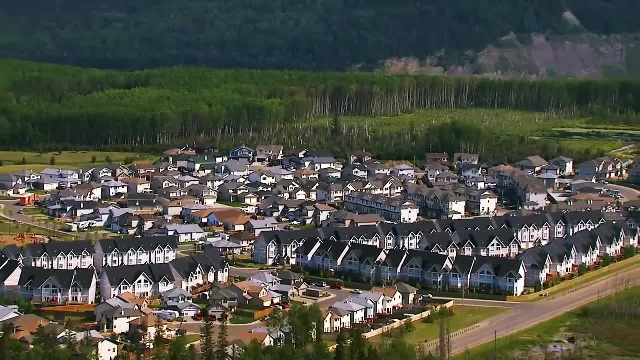 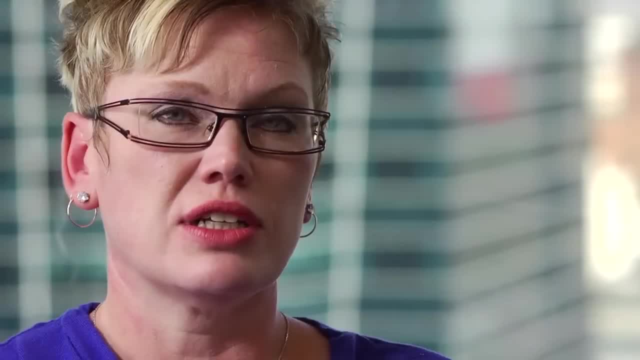 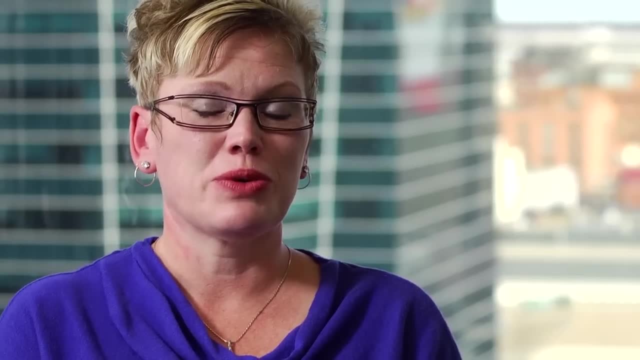 Industry. having certainty is important because we want to continue the investment in our oil sands development. There was a number of issues that were challenging in finding that balance between economic and environmental and social needs. Conserving 22% of Lower Atholabasca did result in trade-offs. 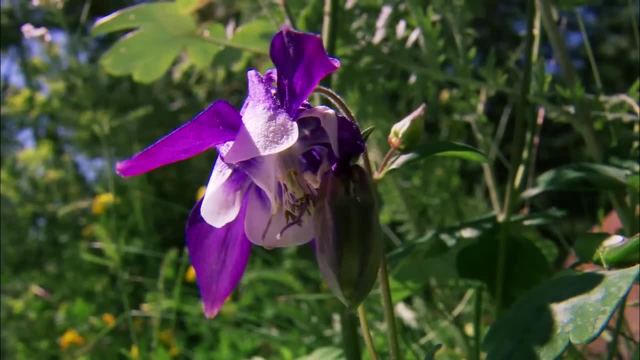 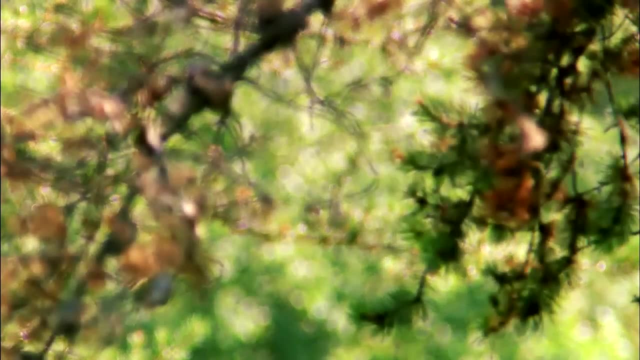 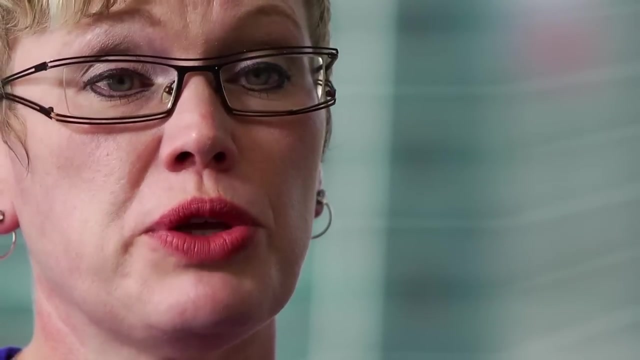 In areas where oil sands will no longer be allowed to be developed. those areas will be managed for biodiversity. That was a significant trade-off for this province. Property rights are not affected under a regional plan. It's very clear in the Lower Atholabasca Plan and will be through every regional plan. 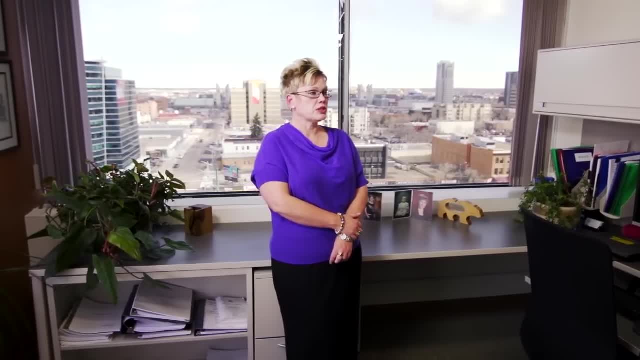 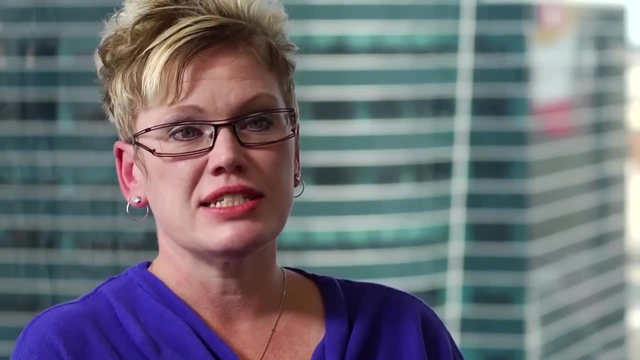 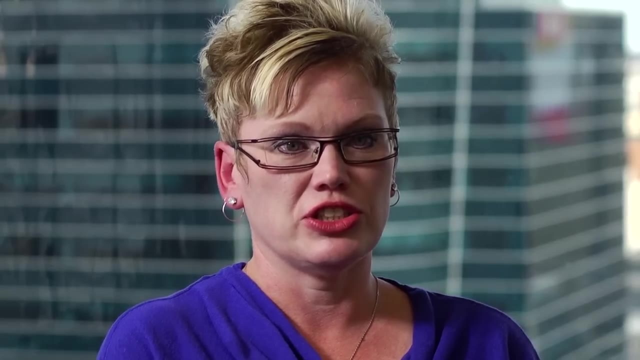 We also are working with Aboriginal peoples to ensure that they are included in our land use planning. I hope a child of the future sees the same beauty that I see in this world. It's things like seeing the rolling fields of Alberta continuing to develop the agricultural industry. 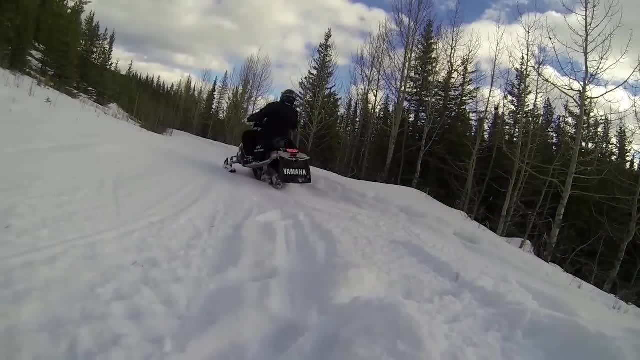 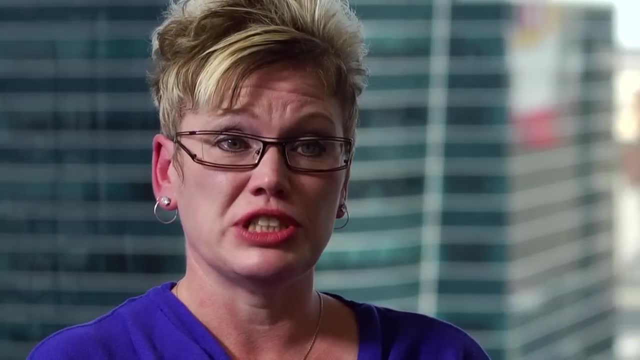 It's reckoned- tourism opportunities throughout many of our provinces and through the parks that we have. It's important as well that the kids paint a picture that includes economic development, which is forestry industries and the development of wood products, and the development of oil and gas opportunities throughout the province. 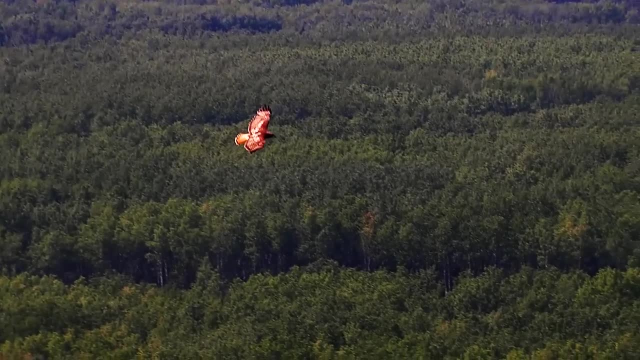 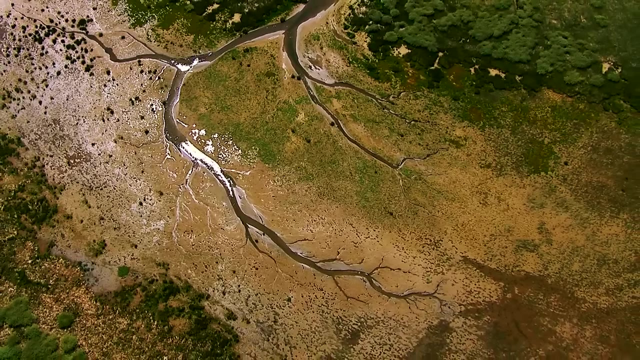 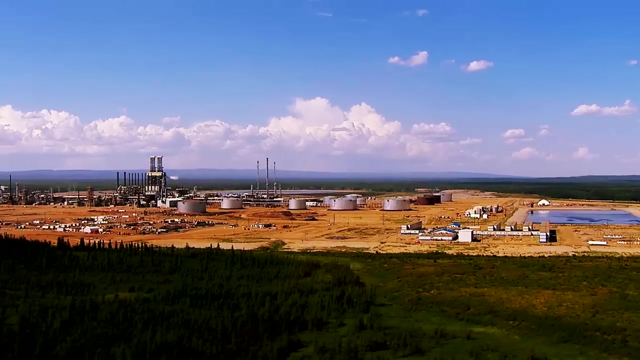 Like Crystal, the Government of Alberta is committed to creating an integrated resource management system that will develop our resources responsibly and sustainably, while protecting our province's environment for future generations. It's an important part of our plan to advance world-leading resource stewardship and shape a sustainable future for all Albertans. 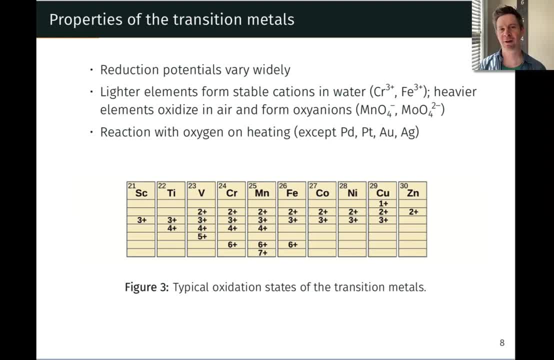 In thinking about the typical charges of the main group elements. they follow patterns that are pretty clear, based on position on the periodic table. Group 1 forms plus 1 cations. group 2 plus 2, group 6: negative 2, group 7: negative 1, so on and so forth. We're not so lucky with the 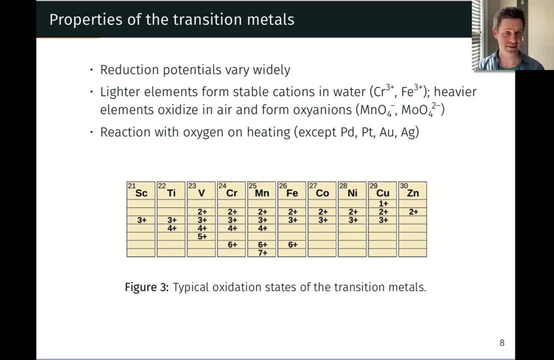 transition metals which can exist in a variety of oxidation states, And most transition elements, I would say, have access to multiple oxidation states: Plus 2,, plus 3,, for example, in the case of iron, Plus 2, plus 3, and even plus 4 in the case of palladium. Copper can be plus 1, plus 2,. 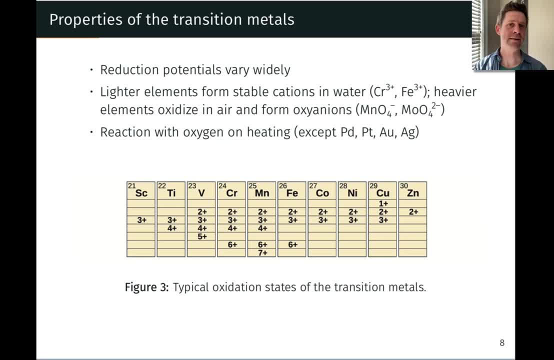 or plus 3.. And this is worth keeping in mind- that different oxidation states of the transition metals give rise to completely different compounds. Copper 1 chloride, for example, is very different from copper 2 chloride. This also means that the reduction potentials of the transition elements can vary widely. 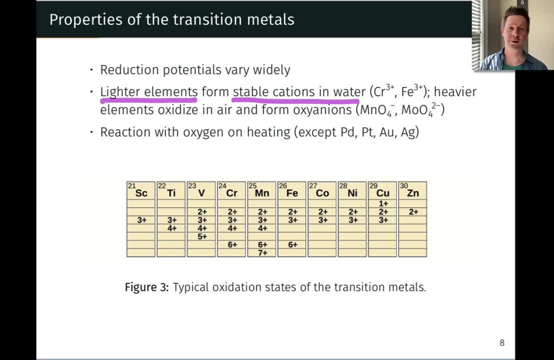 from very good reducing agents to not so good. One thing that we also observe is that different transition elements form different things when they're in water and in air. Generally, the lighter transition elements form stable cations in water. You can take, for example: